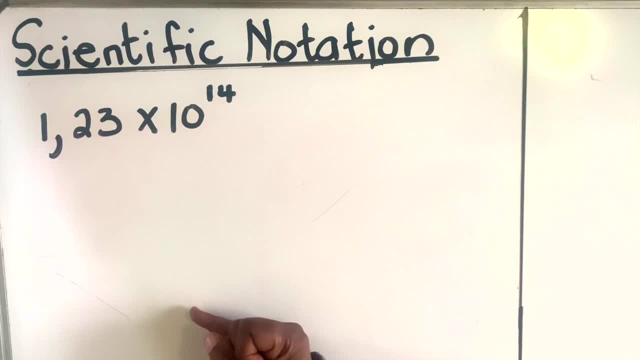 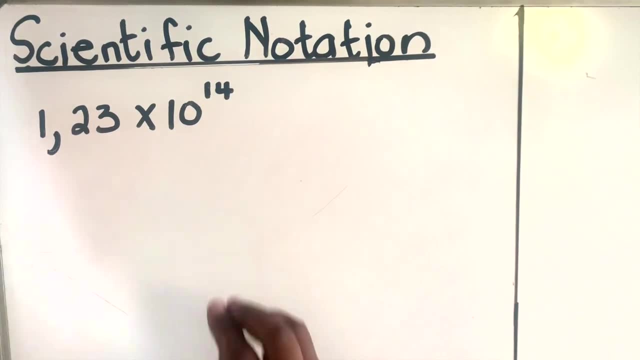 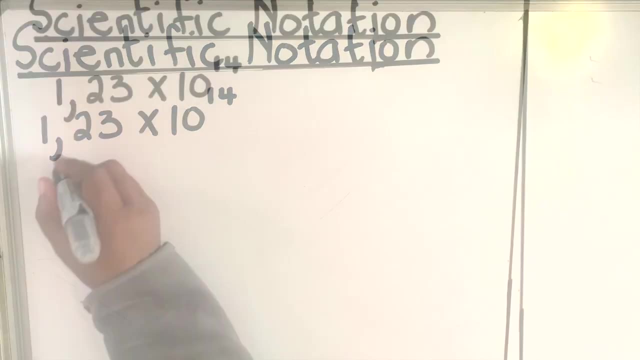 it for us like that: in some question papers they say standard form, in some papers they say decimal form, so you'll see, by having the scientific notation, and then they say: write it in standard form. then they mean, you must take away this times 10 to the powerful. let me show you how we do it. 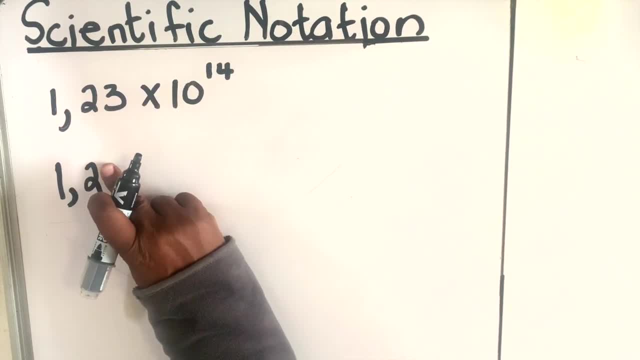 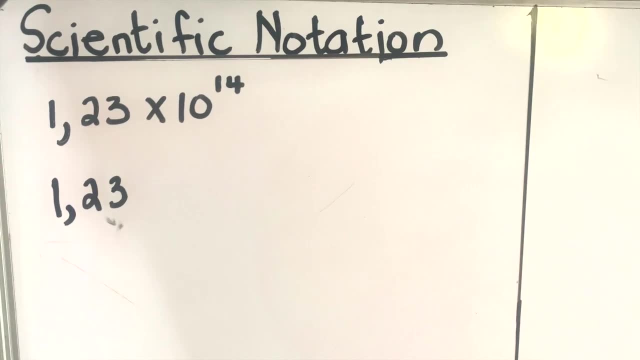 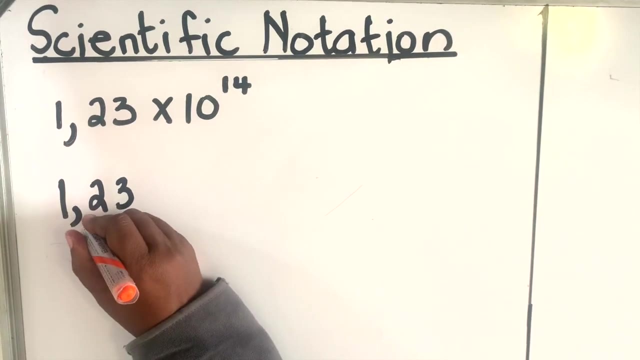 so you're going to move this comma to 3, and then it says times 10 to the power 14.. so what they mean is that you're gonna move this comma to the right 14 times- as many times as the power. so you're going. 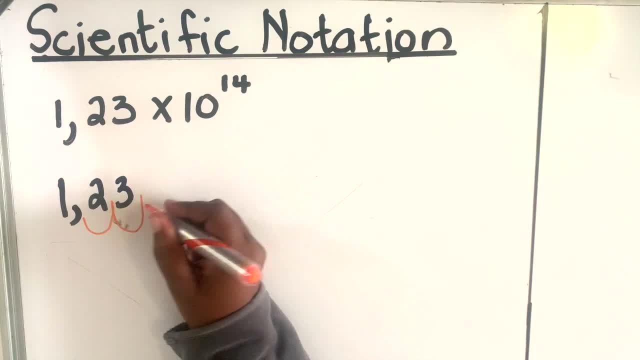 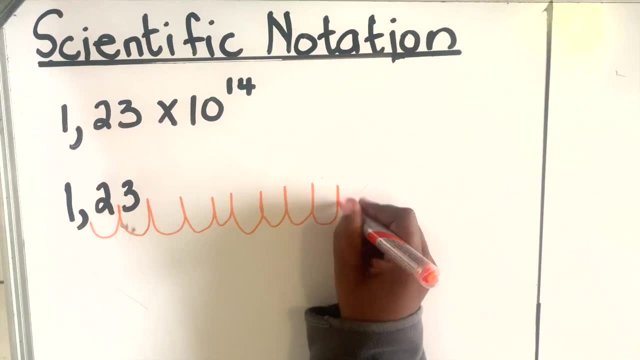 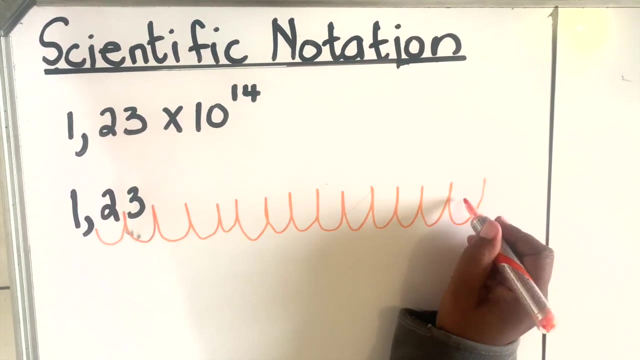 to move the comma from there to there. that's one, then you move it from there to there, that's two, then three, four, five, six, seven, eight, nine, ten, 12, 13, 14.. so the comma will be at the end of the number. what do you put here on these spaces? 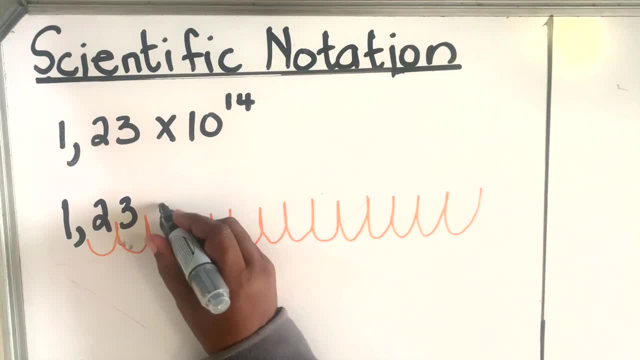 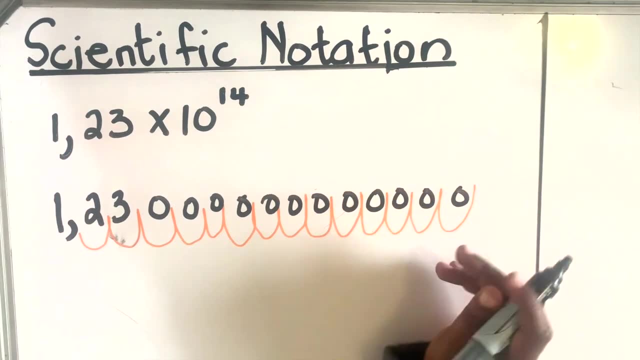 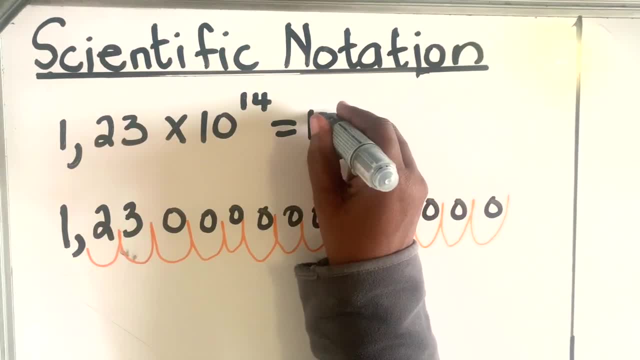 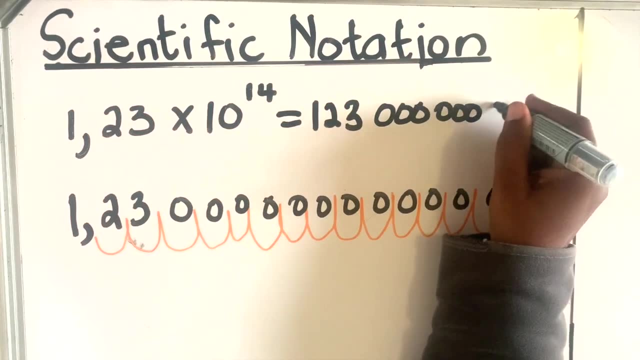 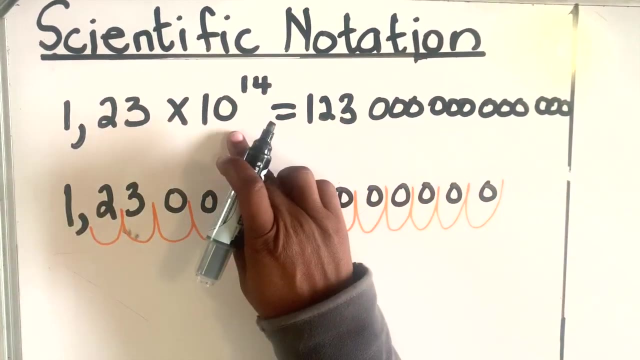 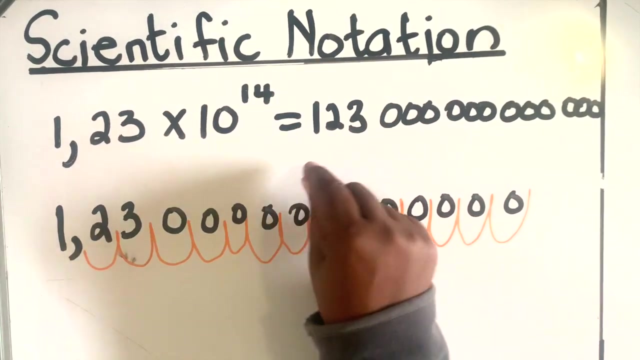 now you go and write your answer. so your answer will be one, two, three and twelve zeros. one, two, three. one two, three. one two, three, three, six, nine, twelve. so this will be the normal notation or the standard notation of the scientific notation that is written. when you look, you do not write 14 zeros. 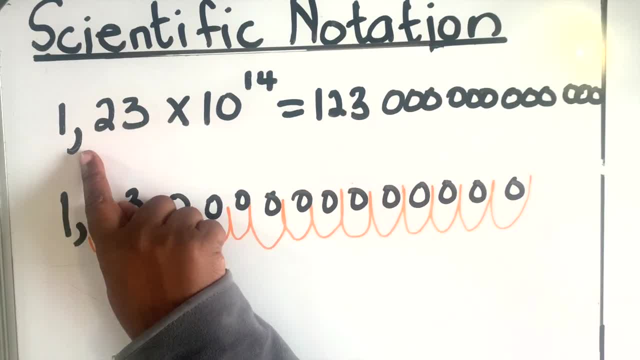 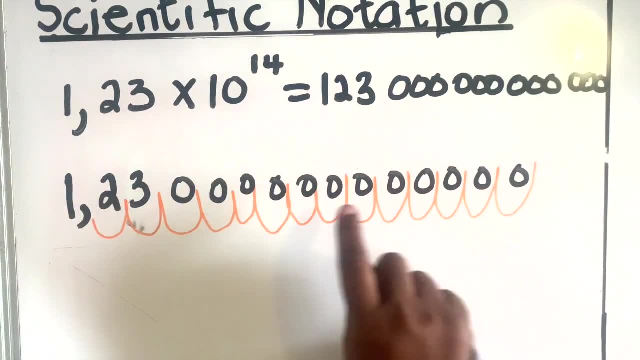 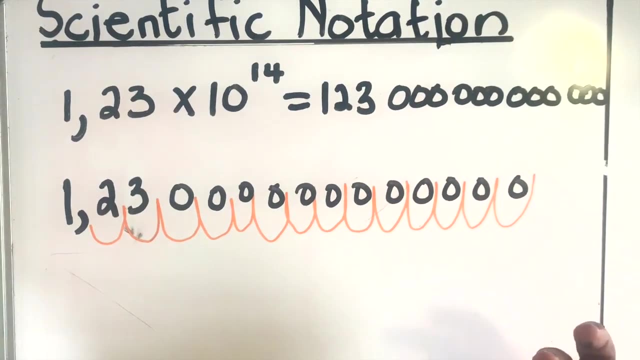 automatically. no, it depends where the comma is. so the comma had two digits. after the comma there's two digits, so you have to move it one, two first, then the other ones are the zeros, so when it's 14, actually going to be 12.. so if you don't want to do it like that, if you get the concept, you can. 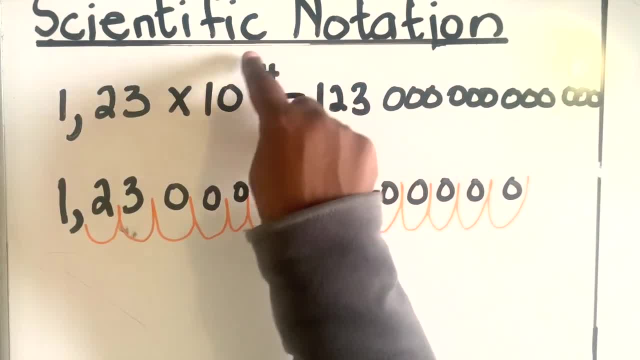 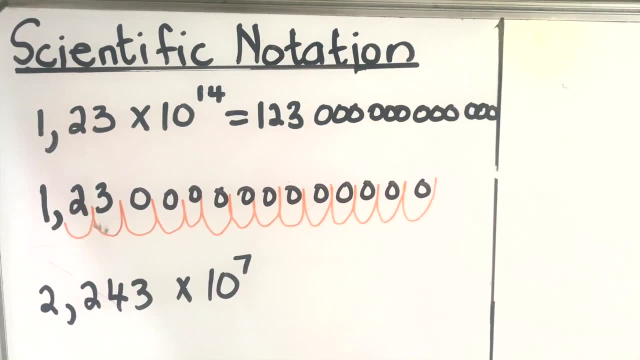 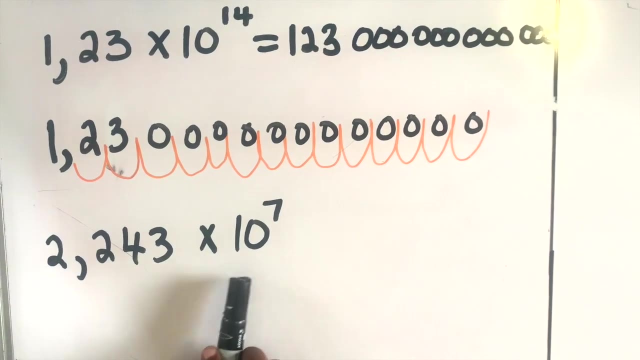 just every time, count the number of digits that you have, subtract them from the power and add that many zeros. let's do it in that method. now, right, with our next example. i'm gonna do it the easier way first, and then i prove it to you that you get the same answer. so here, this is 10 to the. 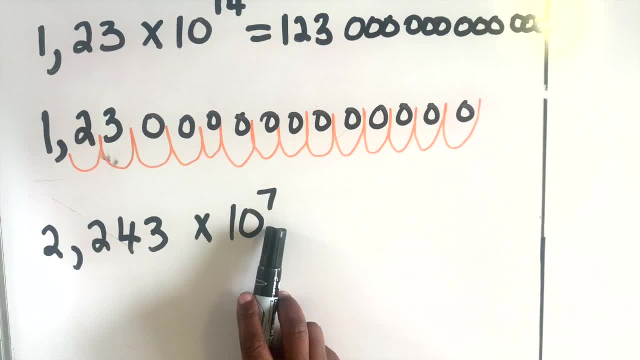 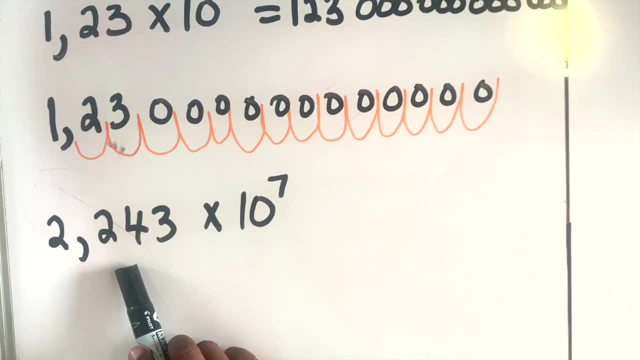 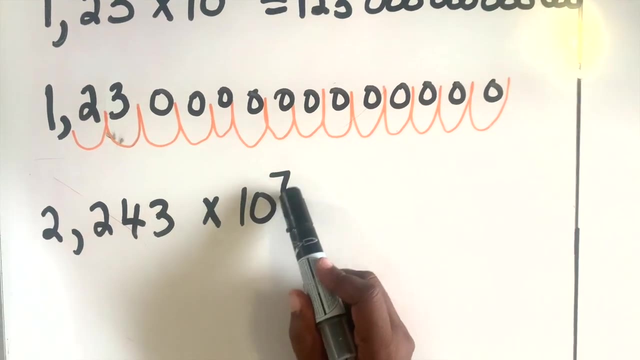 power seven. so you have supposed to move your comma seven times. it does not mean you put seven zeros, it means you move your comma seven times if i count the number of digits after the comma- one, two, three- so i can subtract three here and be left with four. so it means my number will. 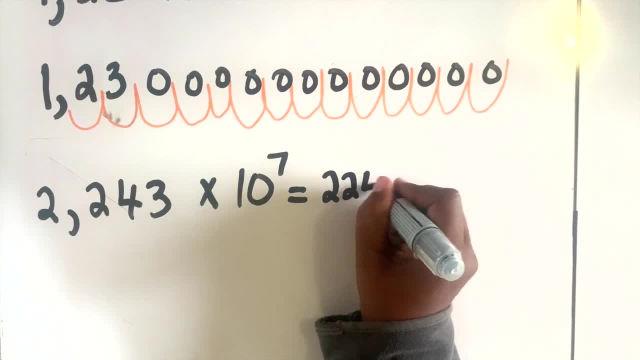 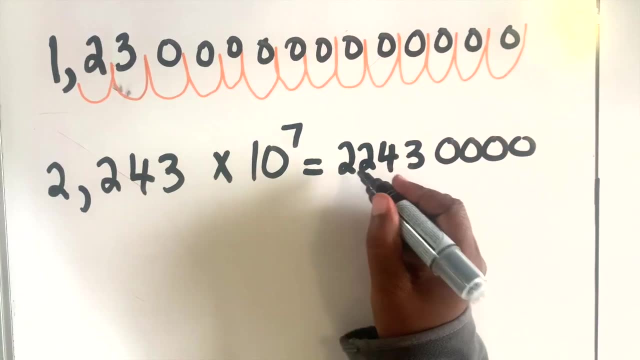 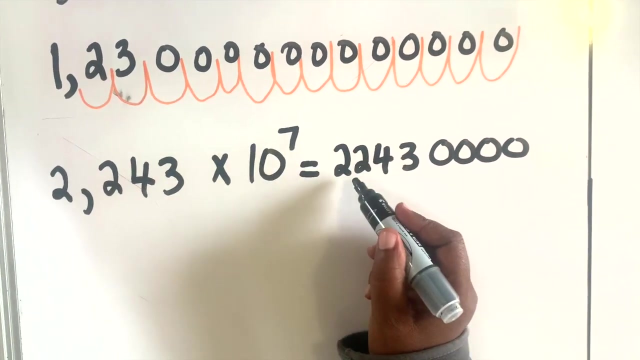 have four zeros. it will be two, two, four, three and four zeros. one, two, three, four. now most learners the mistake that they make: they will keep their comma there. this notation means you move the comma as many times as seven times. so if your answer is two, comma, two, four, three and the zeros, the zeros. 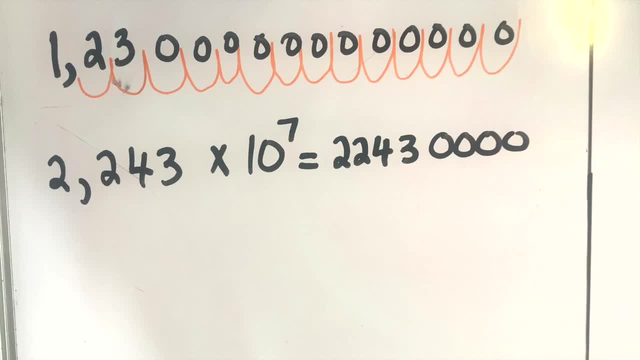 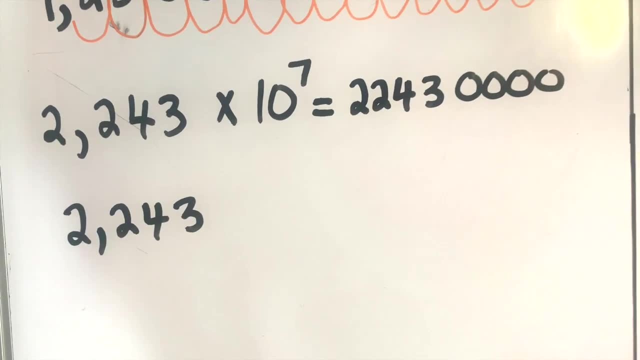 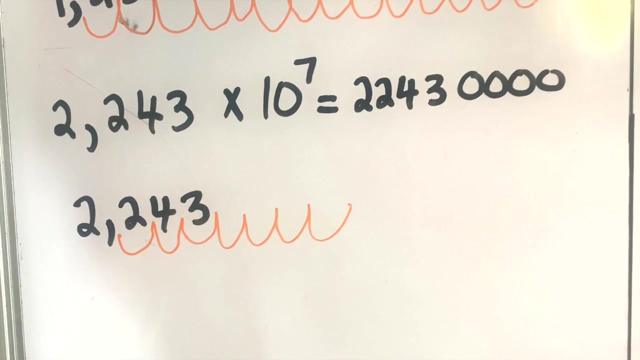 after the comma they don't count. so you're actually making it wrong. so let's switch the the long way. so it's two comma two, four, three. you're supposed to move the zero seven times. so it's one, two, three, four, five, six, seven. so how many zeros must i add? one, two, three, four. 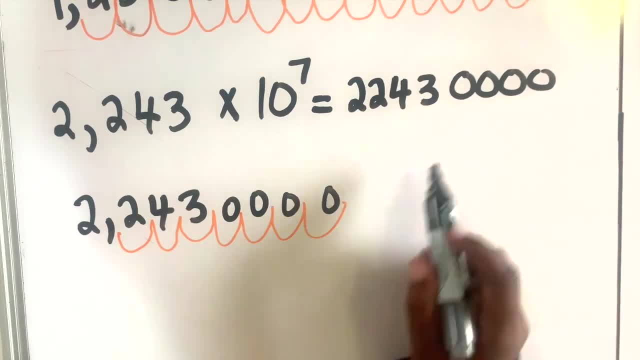 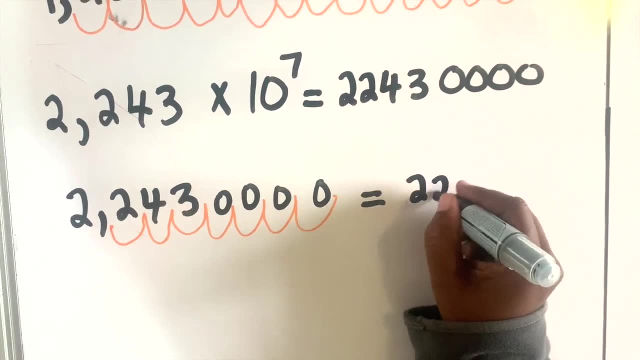 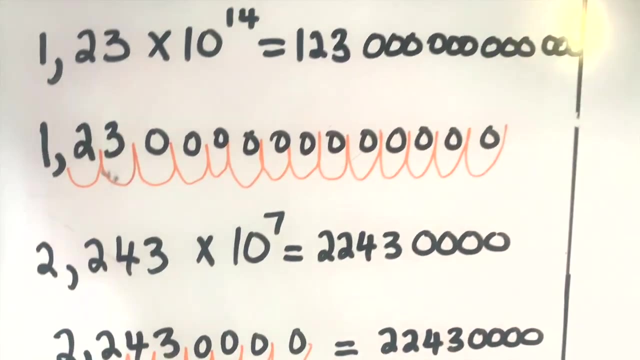 one, two, three, four. so this number is exactly the same as that one, but you have to write it. don't leave it like that. that's wrong. you're supposed to have two, two, four, three and the four zeros. when the comma is still there, it's the same number as the other one. now i want to show you when you are given. 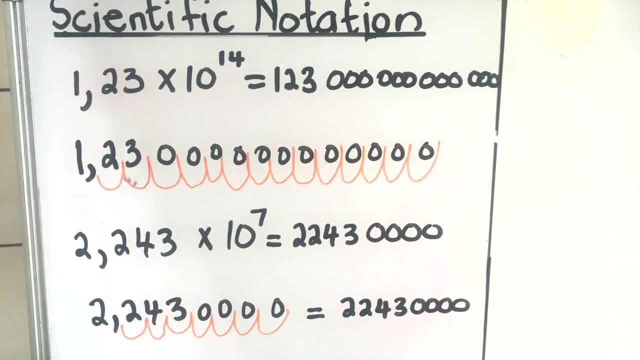 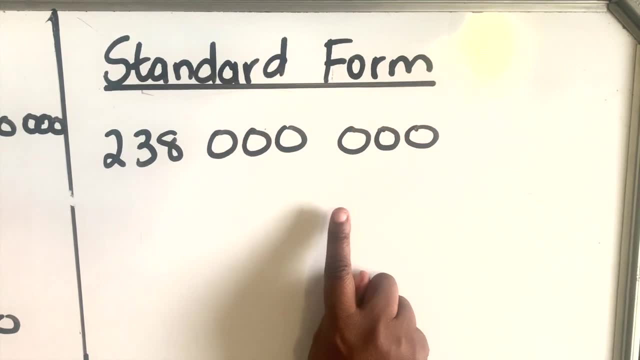 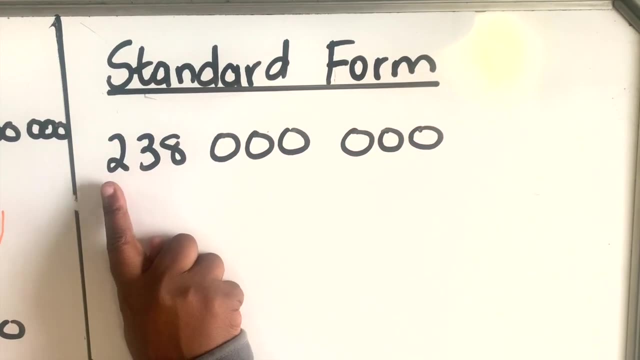 the standard form and the question paper says: write it in a scientific notation. but when we are given a standard form and they say to you, write it in scientific notation, the rule is you're gonna move the comma until one digit. so the comma must be here, it must be two. 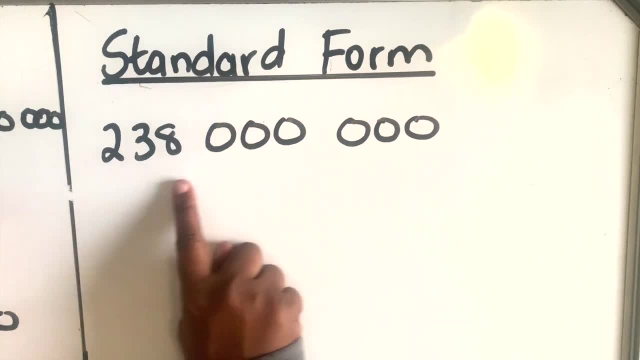 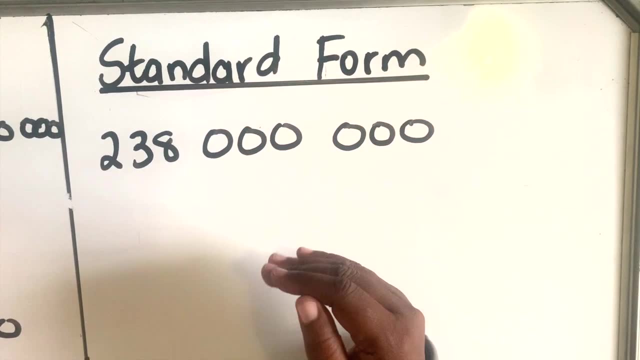 comma. so you move the comma until the latitude. so when you have a number like that, you see there's no comma anyway. so when i say, move the comma, you move the comma from where, if the number doesn't have a comma, there's an imaginary comma at the end. so you're gonna move that imaginary comma. 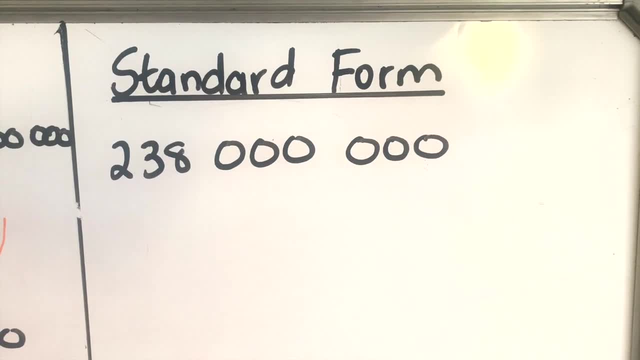 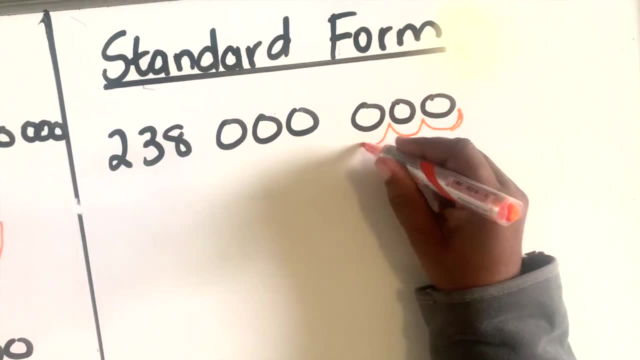 and then every time you move it you count. that is your exponent. so the image of the comma is here. so i'm going to move it until the last digit. so i'm moving it to the left- one, two, three, four, five, six, seven, eight- until one number. 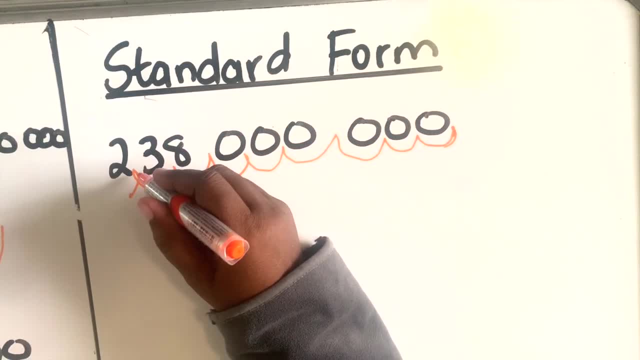 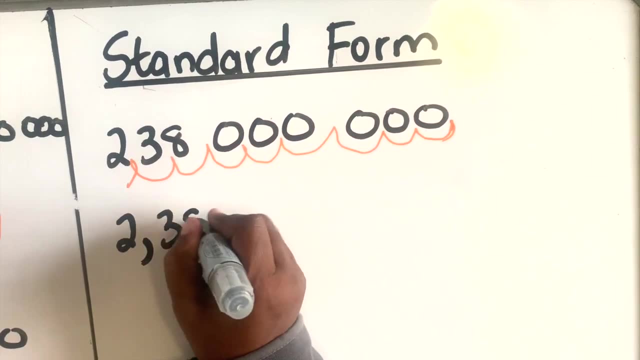 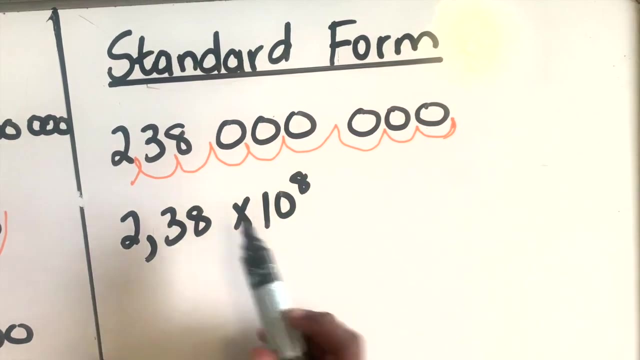 must have one digit, then the comma. so i've moved it eight times. now when i'm writing my number it's gonna be two comma three, eight times ten to the power. how many times did i move the comma to the power? eight. now, when you notice, with this number, 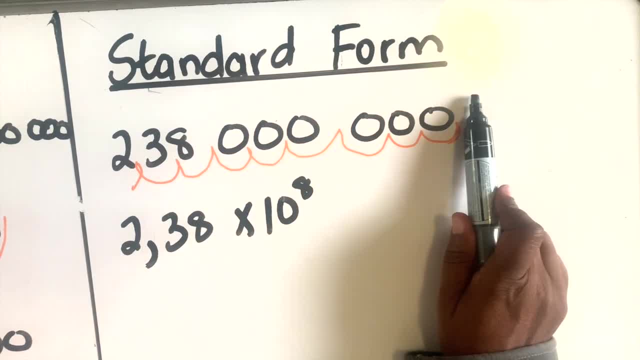 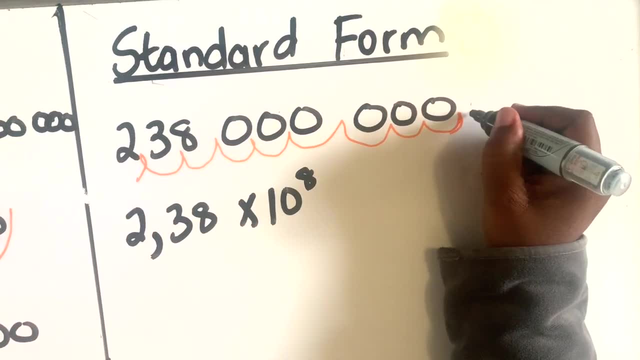 But all these zeros? if you have zeros and there is no number after them, they don't count, You don't write them. You don't write them on the scientific notation. But if I had a one there, I would write all these zeros and the one. 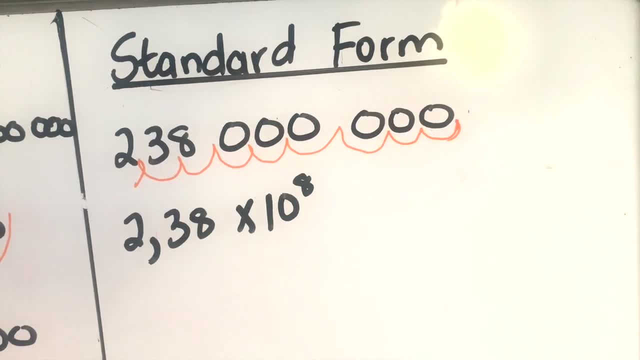 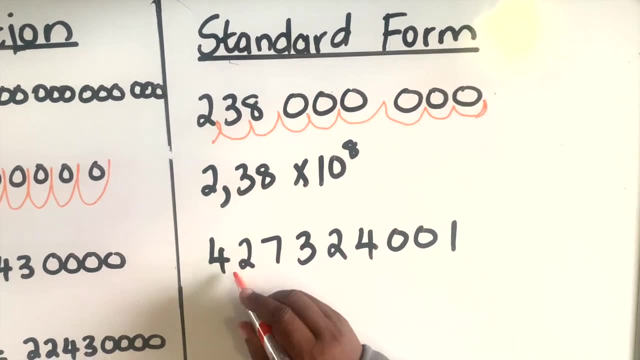 But if it's only zeros with no number, they don't count. You don't write them. Let's look at another example. Okay, with this one we're going to move the comma until one digit, So the comma would be here. 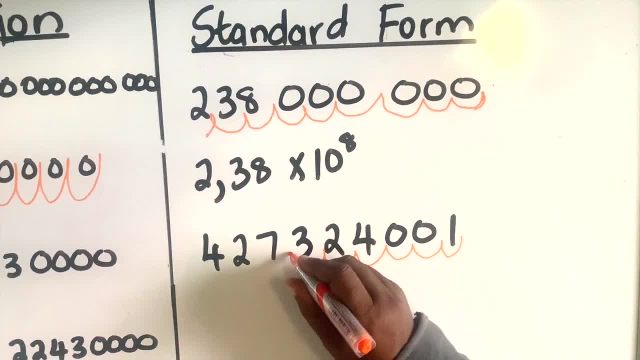 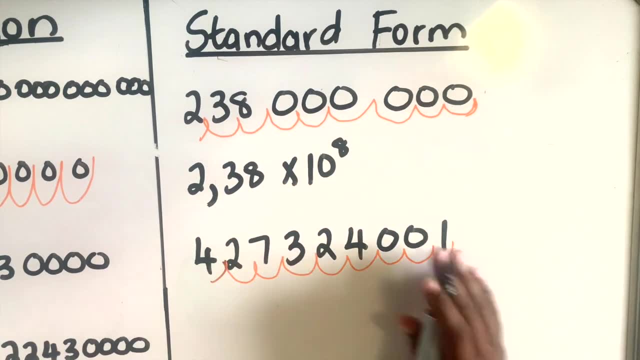 Let's count One, two, three, four, five, six, seven, eight, And so the comma would be there. So when you write, you don't do this in your exercise book, We do it in a script somewhere. 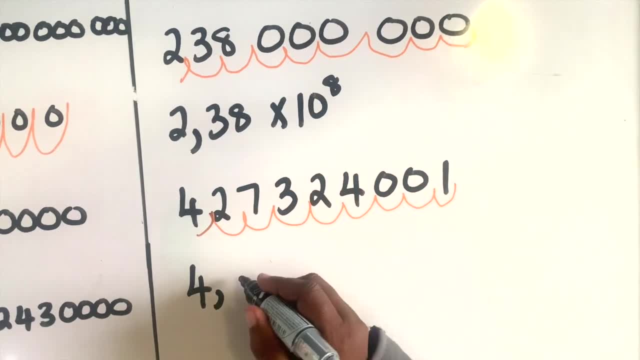 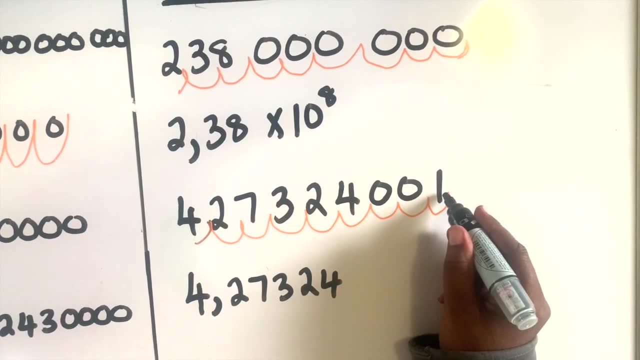 When you come with your answer, you go four, comma two, seven, three, two, four. Now these zeros, you don't throw them away because there's a one after them. So it's zero, zero one. So your answer is like that: 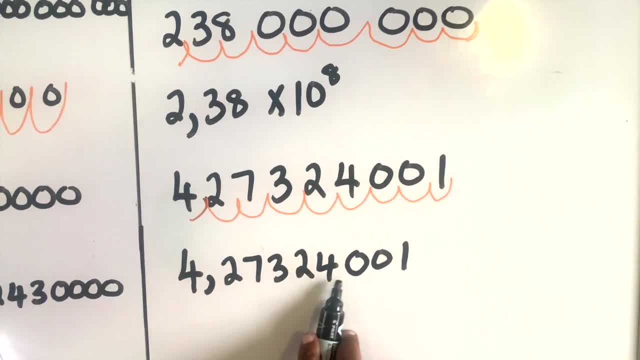 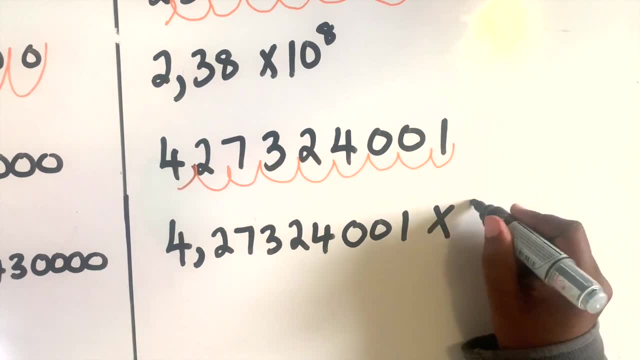 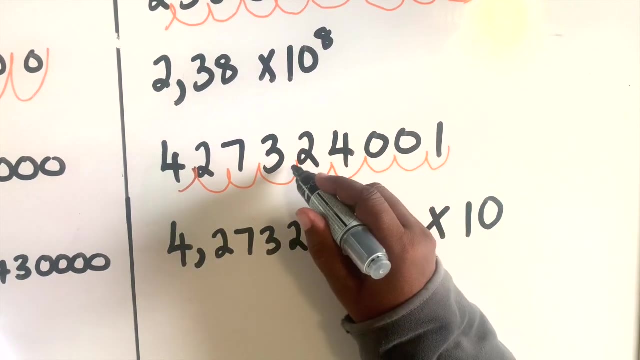 It's two comma two, seven, three, four, four, zero, zero, zero one, But this number is very small, So something It's missing. The missing part is times ten exponent. How many times did you move the one, two, three, four, five, six, seven, eight- to the power eight? 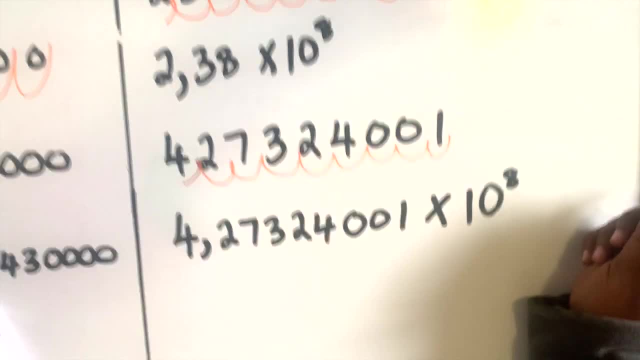 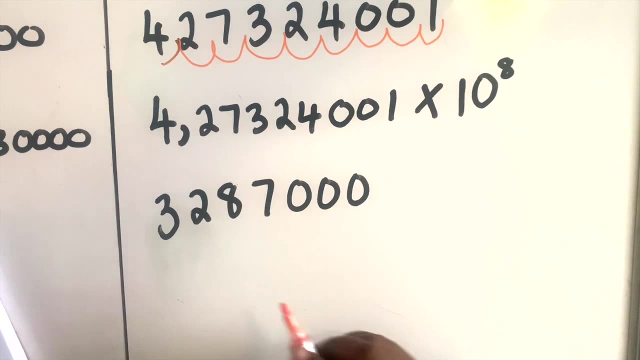 Okay, My example was not good. It doesn't mean every time is to the power eight. Okay, let me do another one. It's not to the power eight, Right? Let's look at this example. How many times am I going to move until I have one digit before the comma? 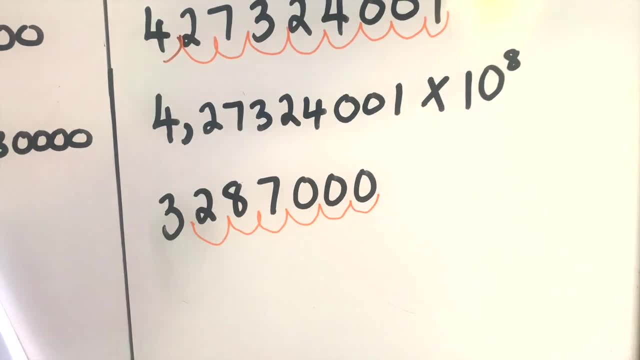 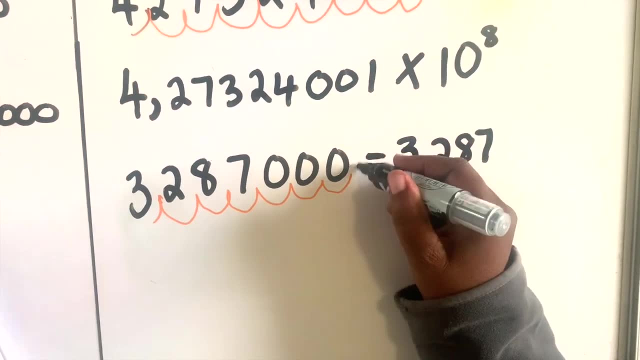 One, two, three, four, five, six. The comma will be there, So my answer will be three comma two, eight, seven. There is no number after this zero, So I don't need to add them. Times ten to the power. 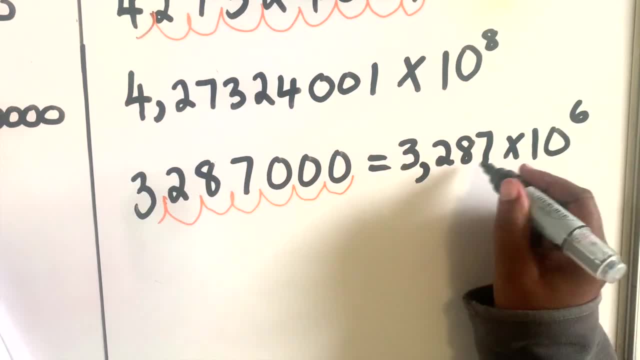 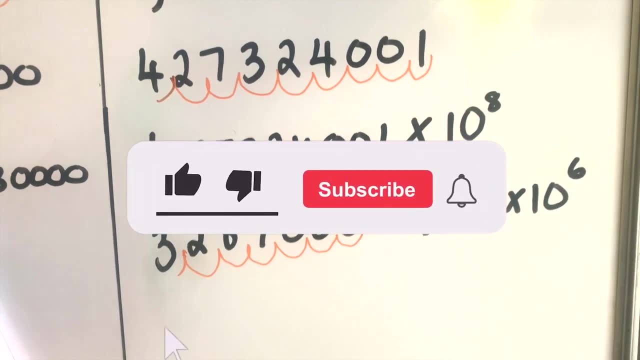 How many times did I move the comma Six- So it's times ten- to the power six? This is how you do scientific notation. Please practice. Practice is not something that is hard. You just need to practice it and then you'll get better. 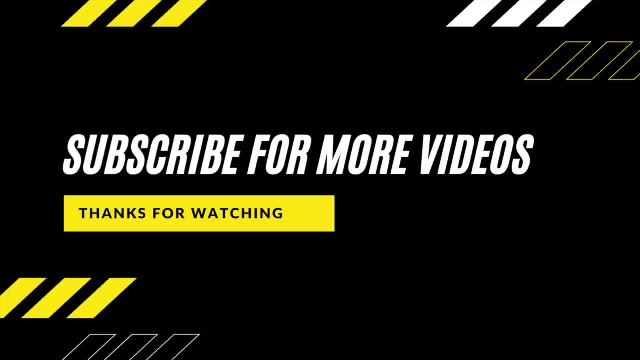 This is the end of my lesson. Thank you for watching. Thank you.